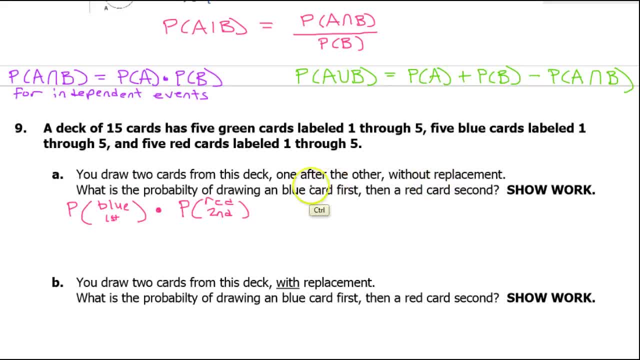 they don't say the word red, they don't say the word green, they don't say the word, and you can read it. as we're going to draw a blue card and then a red card, It's really an AND problem. Okay, now pay attention to the fact that we're not 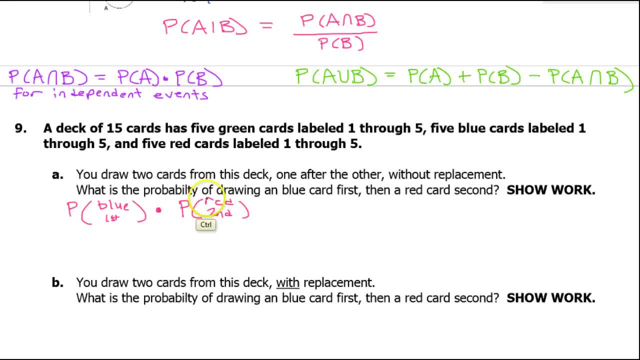 putting the first card back. So the second probability will change a little bit. So what is the probability of drawing that first blue card? Target over total is how we do probability. There are 15 cards in the deck, so right from the start. 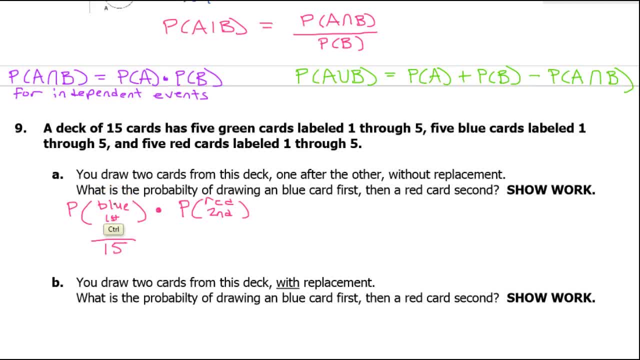 the total is 15.. We're trying to draw a blue card. Well, there are five blue cards right from the start, so that probability is five out of 15.. So next we have the probability of drawing a red card. but be careful- without replacement. So we did not put the blue card back, so that means 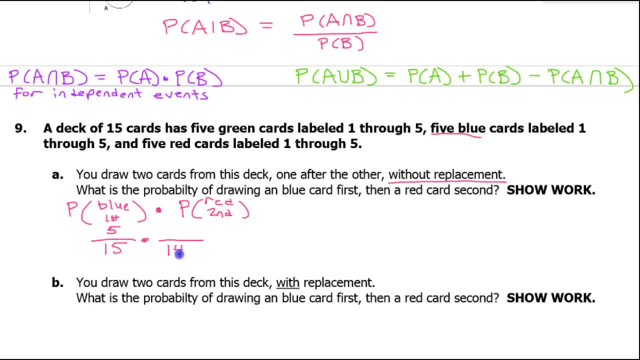 we don't have 15 cards left anymore Now there are only 14.. However, we drew a blue card the first time, so we didn't take any of the red cards away, so there are still five red cards. so there are five red cards out of a total of 14 cards. so if 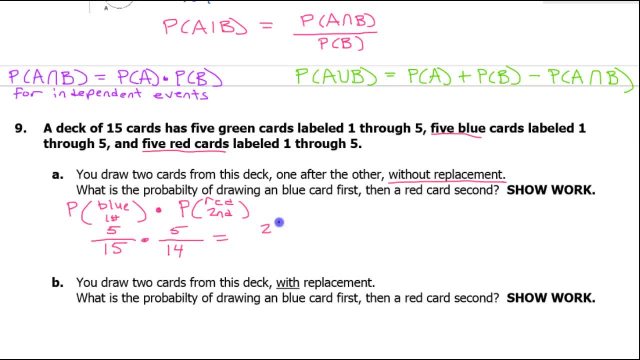 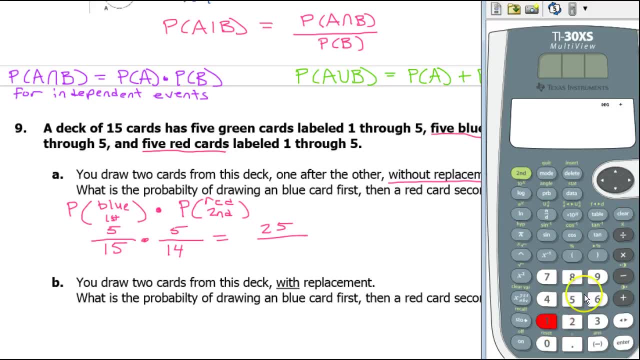 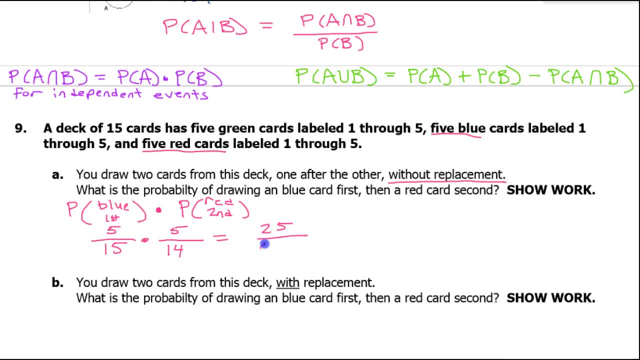 we multiply these together, that's going to be the probability. so this will be 25 out of whatever is 15 times 14, okay, 210, and this number does reduce, but i'm going to let you do that on your own. now you draw two cards from this. 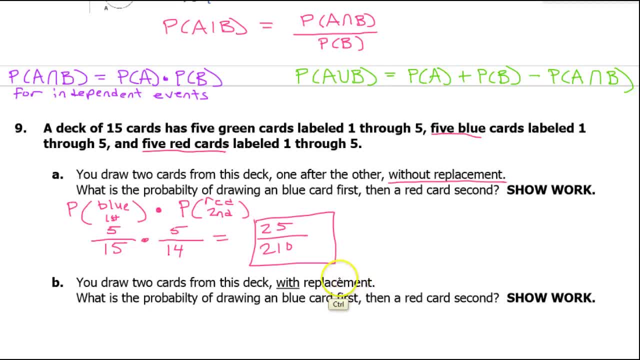 deck with replacement. so this time we're going to draw a card, put it back and then you stop. we'll go and close and quit. this time we're going to go and then we'll go and forgive. but if, before we're done, we start it over, so we do. 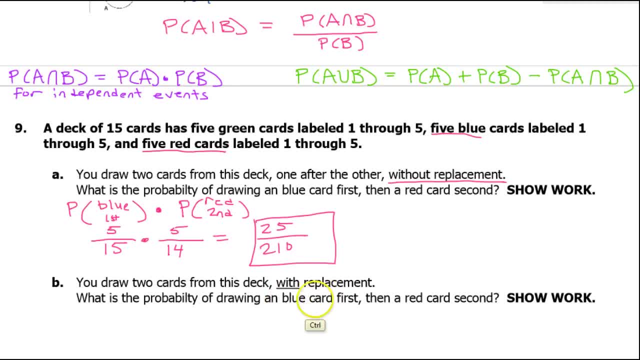 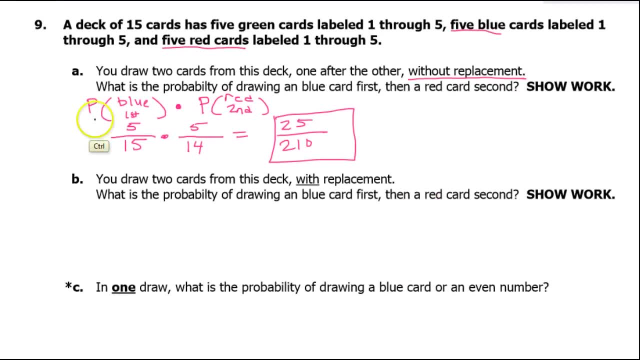 we get two of these three, four codes- got to think about a lot of propor prisoner- then draw the second card. What is the probability of drawing a blue card first and a red card second? Alright, so it's the exact same situation. So this is again an AND problem. so we're. 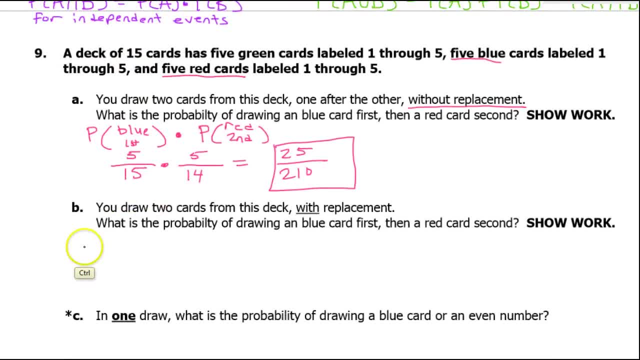 going to use the AND formula. So I'm still going to calculate the probability of drawing a blue card first and I'm going to multiply that times the probability of drawing a red card second. Okay, but we're putting the card back. we're putting the first card back, So 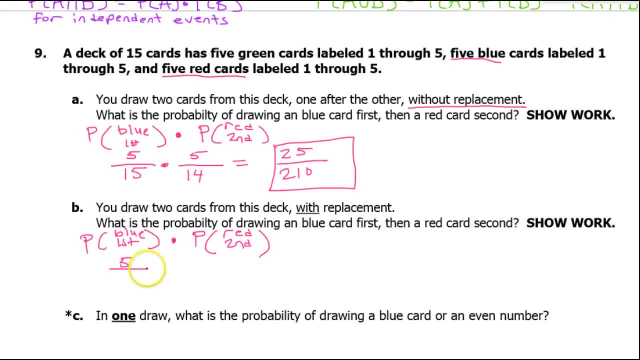 the first fraction will be exactly the same. I have five blue cards out of a total of fifteen, So the only thing that's going to change is for the red card. I have five red cards and the total is still going to be fifteen because with replacement we put 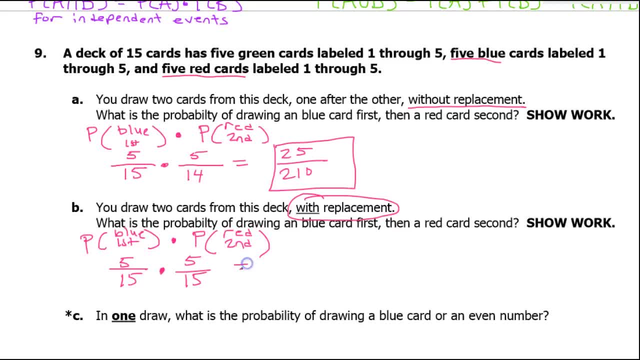 the first card back, so we have a total of fifteen again. So this is going to be twenty-five out of two hundred and twenty-five. Okay, so if you chose to reduce those like five out of fifteen, that would have been one out of three and then times one out of three. 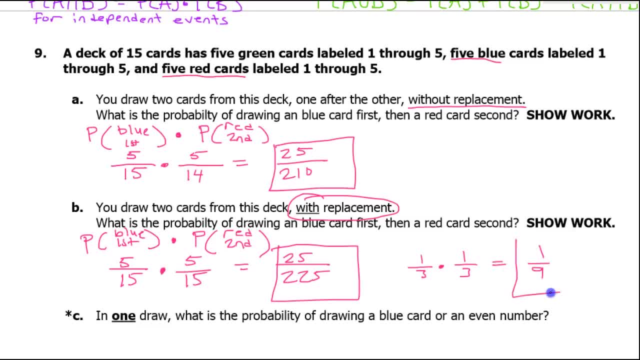 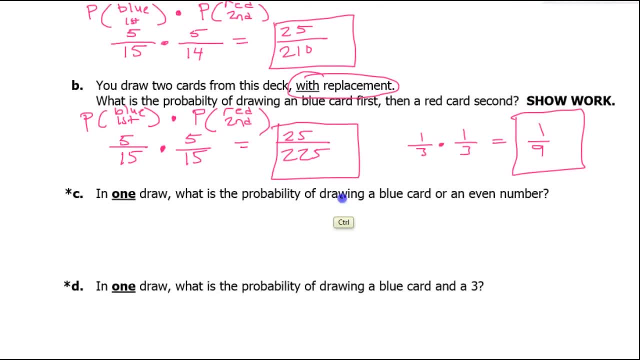 so that would have been one out of nine, So maybe you did it that way. Now, in one draw, what is the probability of drawing a blue card OR an even number? So obviously this is an OR problem, so I'm going to use 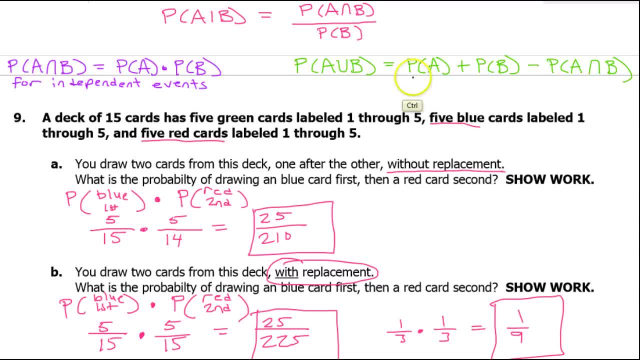 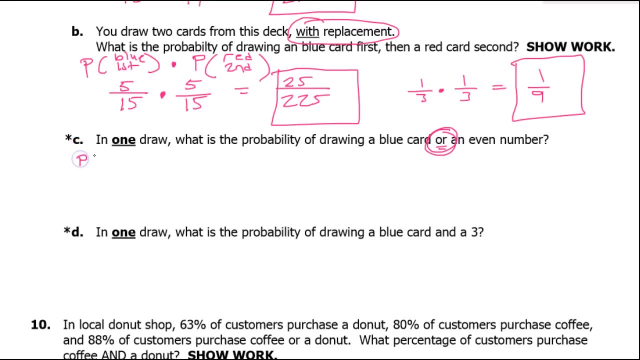 the OR formula. Okay, so check this out. I'm going to be using this formula right here: Probability plus probability minus the overlap, which is what that is. So let's see blue card. So I need to calculate the probability of drawing a blue card. Okay, 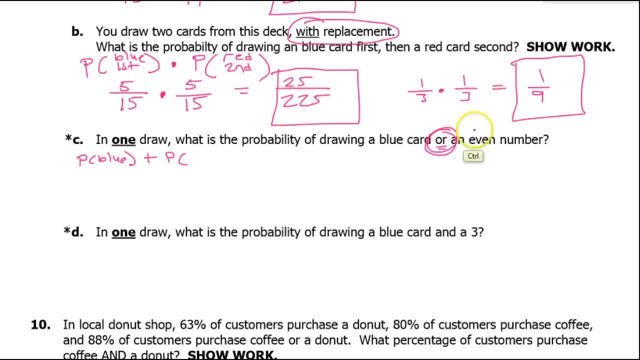 and I'm going to add the probability of drawing an even number, and then I'm going to subtract the probability of drawing blue and even. Okay, so this is in one draw. So how many blue cards are there? Well, there are five. 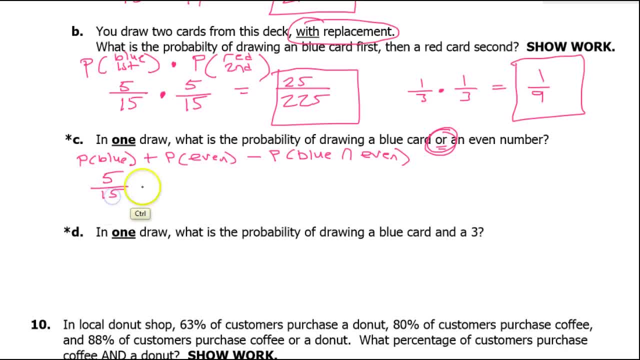 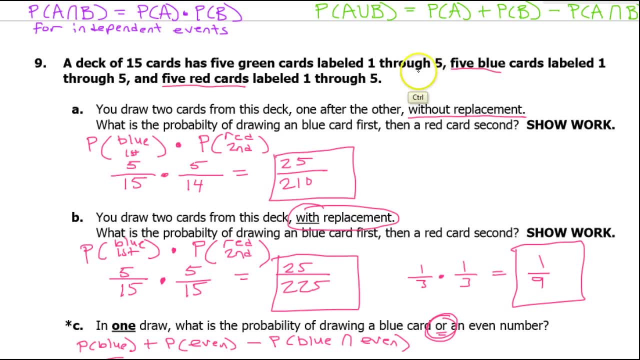 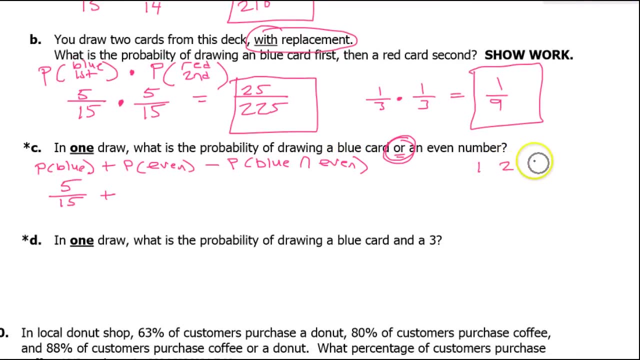 blue cards out of a total of fifteen. Okay, how many even cards are there? Well, they're all numbered, one through five. okay, So just picture this for a second. So I've got one, two, four, Okay, only one blue. 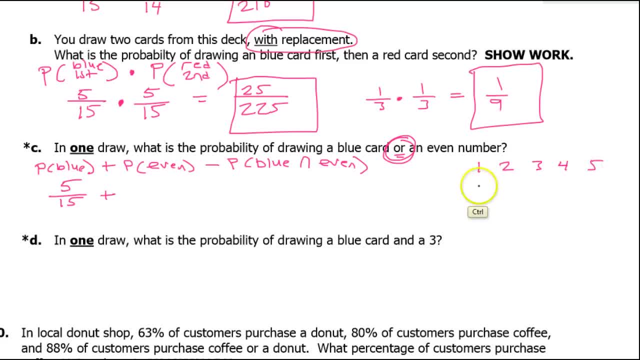 So one plus two equals, One plus two equals three, Two plus five equals. I put into the ум sabia and that's a positive, but I'm going to say zero, 1, 2, 3, 4, 5, and this repeats 1, 2, 3, 4, 5, okay, so how many even numbers are there? 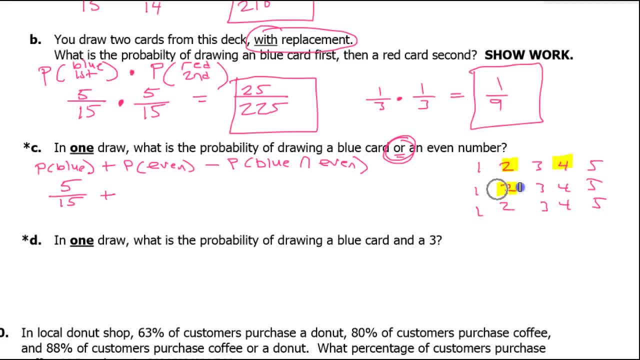 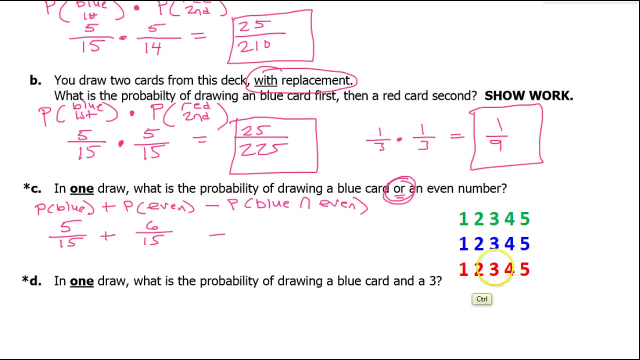 Well, there are. these are the even numbers, would be like right here. so there are 6, there are 6 even numbers out of a total of 15,. alright, so probability of even is 6 out of 15,. okay, I decided to break down and go ahead and draw a visual representation of 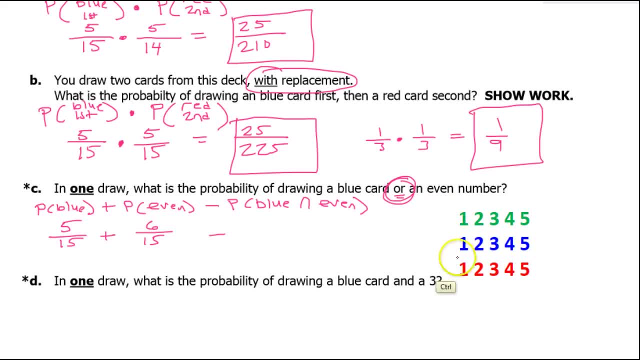 my deck showing my 5 green cards, my 5 blue cards and my 5 red cards. So, because this next part is the trickiest, I need to see the probability of pulling a card that is blue and, even so, how many of those are there. 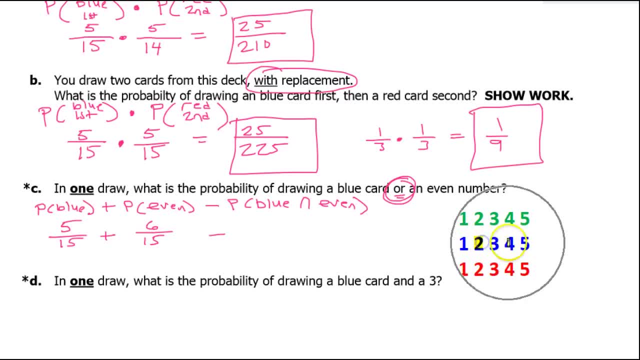 Well, here are my blue cards, and how many of these are even Boom boom. so I have 2 cards out of the 15 are blue and even so, that is going to be the final fraction. So I just need to calculate this, so I have like denominators. so I am really looking. 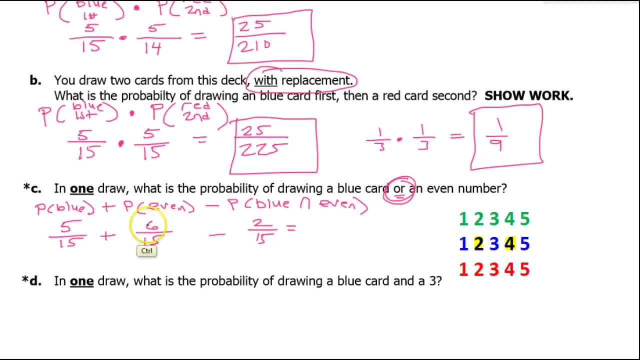 at the numerators: 5 plus 6 minus 2,. 5 plus 6 is 11, minus 2 is 9, so that is going to be 9 out of 15,. okay, so that is going to be the probability of drawing a blue card. 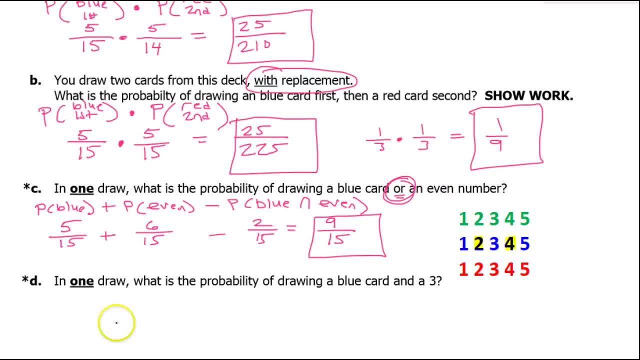 blue card or an even number or another way I could have done it. if I am going to take the trouble to draw a diagram, I could just use the diagram to answer the question. so blue, or even I could highlight all the blue numbers: okay, 1,, 2,, 3,, 4,, 5, now, or is more? 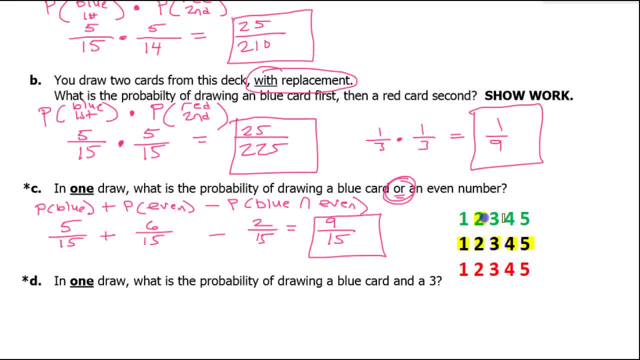 so, in addition to that, I could highlight all the even numbers: Boom, boom, boom boom. so that is 5,, 6,, 7,, 8,, 9, so that is 9 numbers, 9 out of 15,. 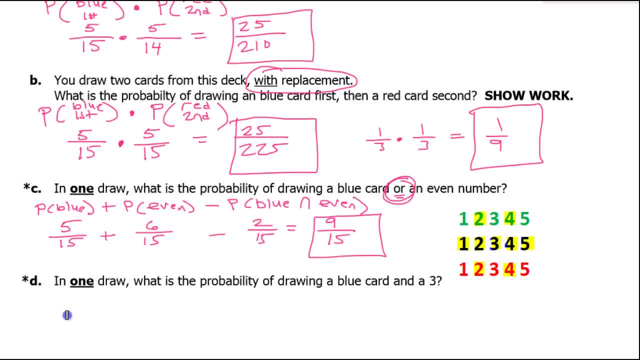 so if I am going to make the diagram, I could have just used the diagram Now in one draw. what is the probability of drawing a blue card and a 3?? Well, this is an and problem, so I could use the and formula. 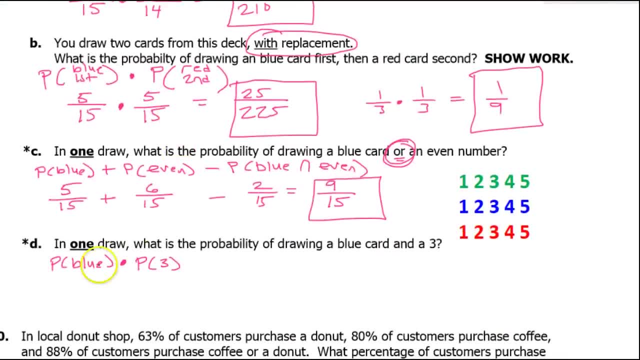 So I can find the probability of blue. alright, there are 5 blues out of a total of 15, times the probability of drawing a 3.. Well, there are 3 3s out of a total of 15, so if I multiply that out, that is going to. 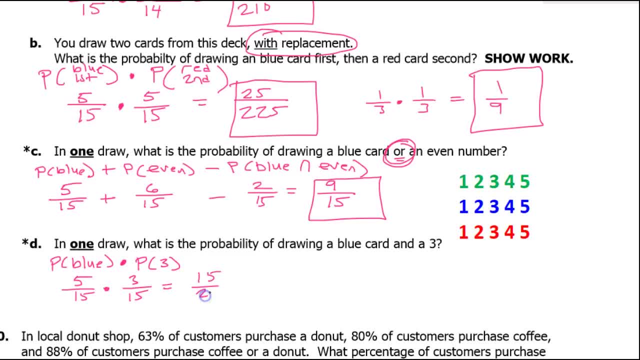 be 15 out of 200.. Okay, So this is 200 and 25.. Okay, Now this reduces down to 1 out of 15,, by the way, Okay Now, I did not need the diagram for that, I could just using the words of the description. 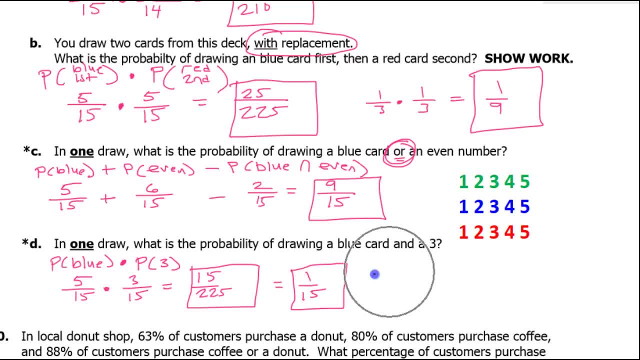 I could have found these two probabilities. I did not need a diagram. Now, if I have the diagram, which is not hard to make, then I could have used the diagram to answer the question. So the probability of drawing a blue card in one draw. 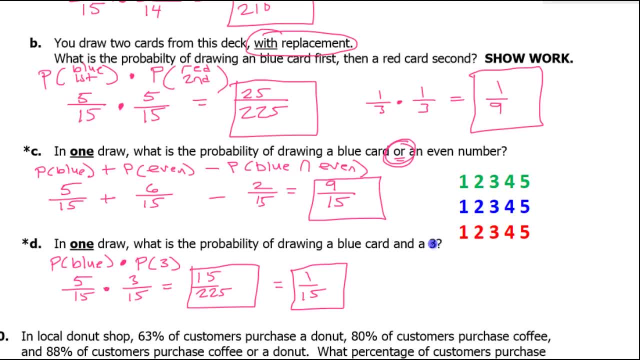 drawing a card that is blue and a three. well, that's a long way of saying a blue three. So how many blue threes are there in the deck? Well, guess what? There's one blue three. So that's the target, out of a total of 15 cards. 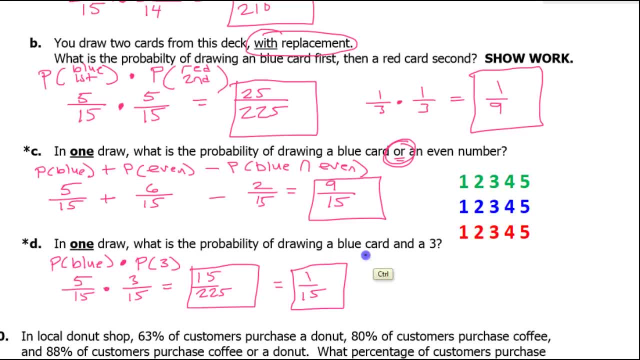 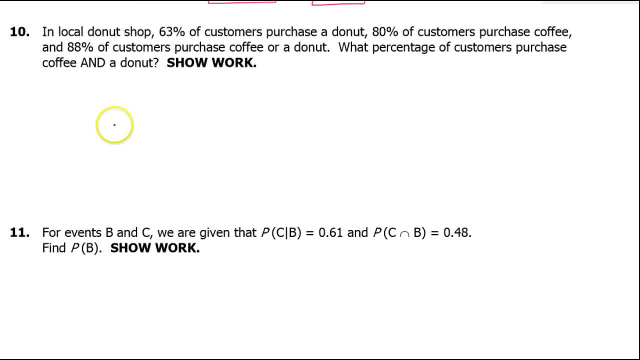 So if you have the diagram, you can quickly see that it's going to be one out of 15.. All right, for these last few problems we will definitely have to use the formula because we have no diagram Now. in a local donut shop, 63% of customers purchase a donut. 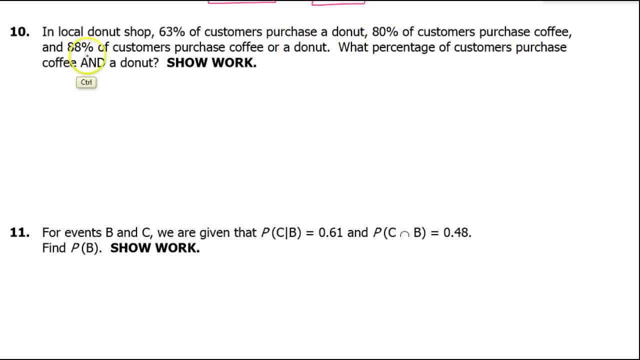 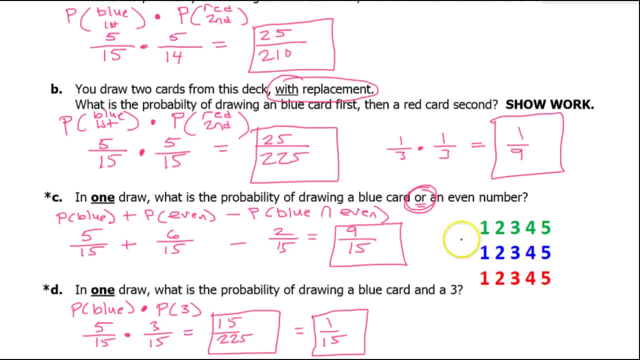 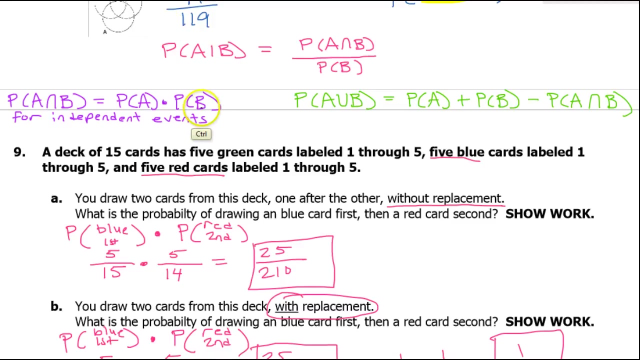 80% purchase coffee. 88% purchase coffee or a donut. What percentage of customers purchase coffee and a donut? Well, first we have to decide which one of these three formulas we're going to use. Now, all of the formulas mention, and so that's not going to help us. 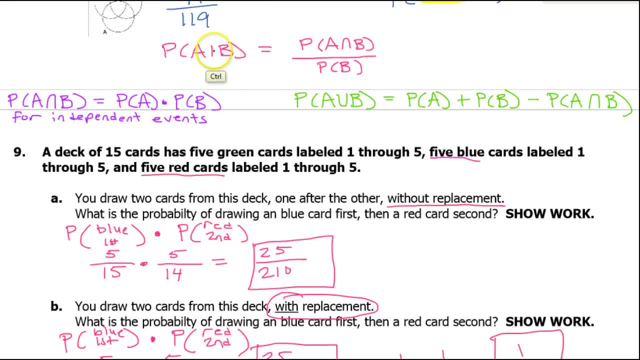 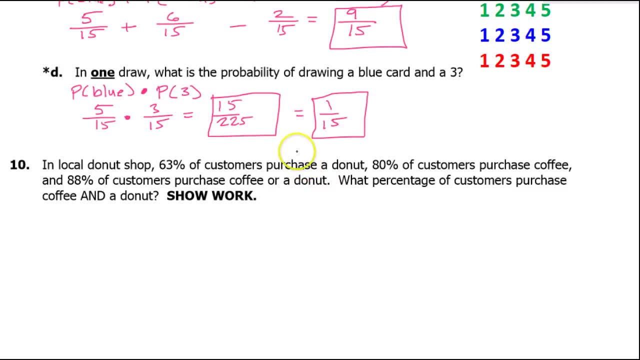 However, this red formula is the only one that has given in it and the green formula is the only one that has or in it. So if this problem mentions given, or if it mentions or, then I will know which formula to use. 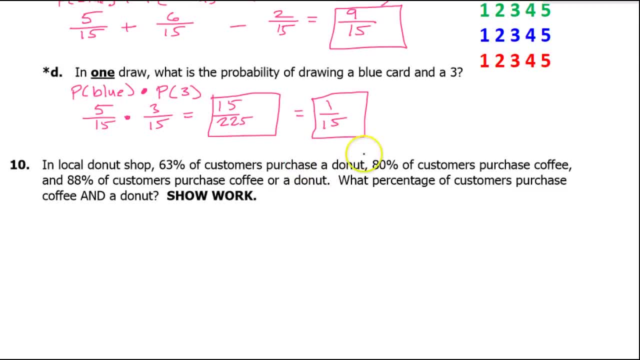 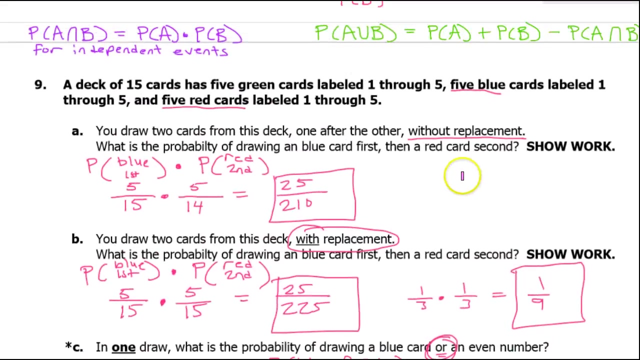 If it doesn't mention either of those, then it's probably the and formula. But look what I see right here. Okay, 88% of customers purchase coffee or a donut. Okay, you see the or right there. That tells me that I'm going to use the formula. that looks like this: 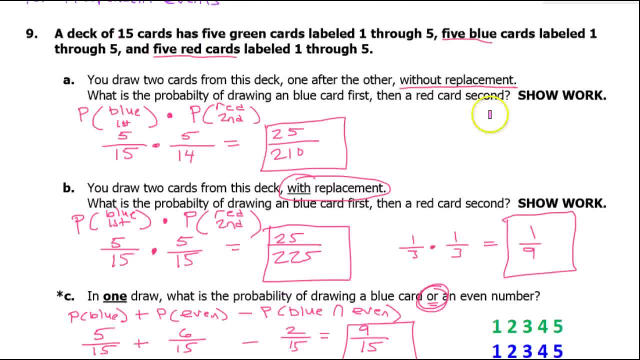 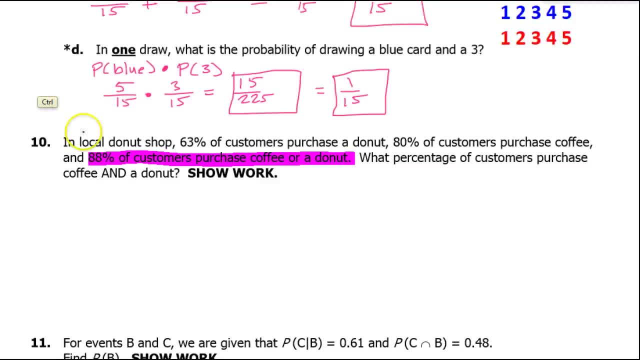 Okay, so I'm going to use this green formula right here. Now, instead of A's and B's, I need a new set of events. So let's let D represent eating a donut. We're going to let C represent drinking coffee. 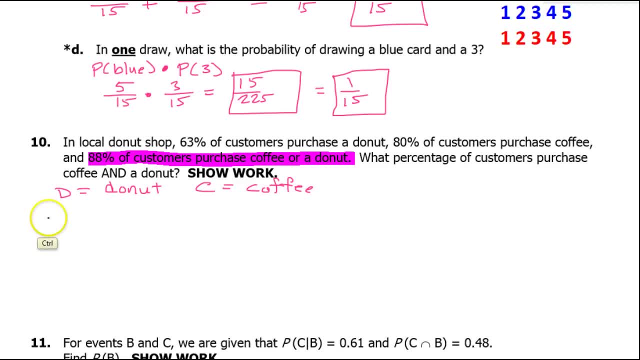 So, with that in mind, the or formula becomes: the probability of D or C is going to equal the probability of D plus plus the probability of C minus the probability of D and C. Okay, okay, So let's hunt through the problem and see what we know. 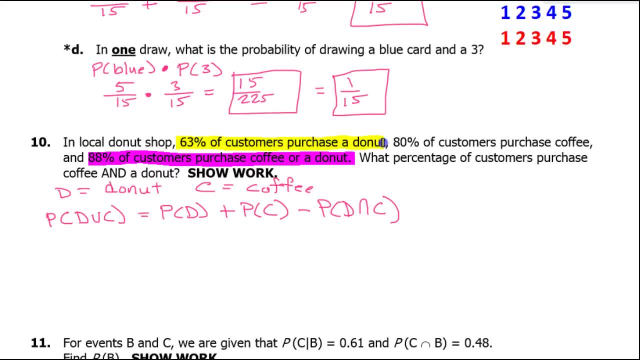 63% purchase a donut. Okay, so that's the probability of D. I'm going to go ahead and write these probabilities as decimals, So I know the probability of D is 0.63.. All right, 80% of customers purchase coffee. 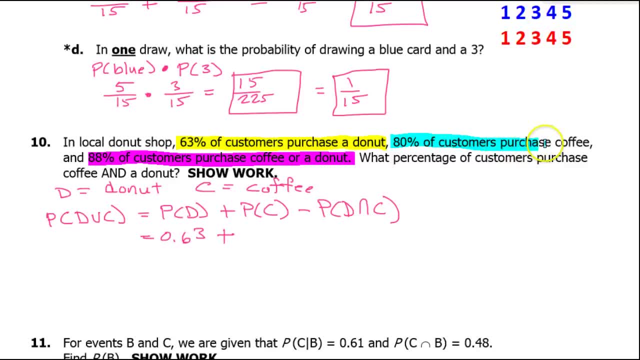 So that's another event. All right, that's the probability of C And I will write it as 0.80.. 0.80%, Okay. next we have the probability: 88% of customers purchase coffee or donut. 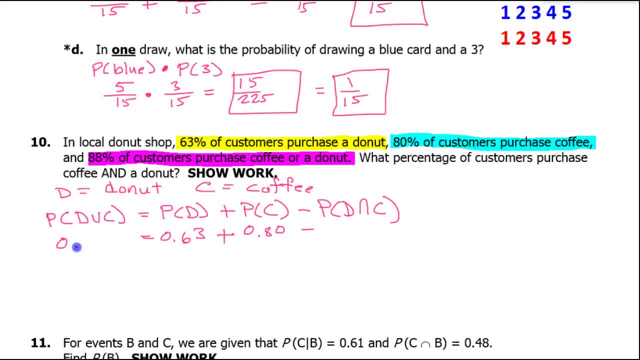 So that's right out here in the front. That is 0.88.. All right, coffee or donut. So that just leaves the probability of purchasing a donut and coffee. That's what we're looking, So I'm just going to leave this alone. 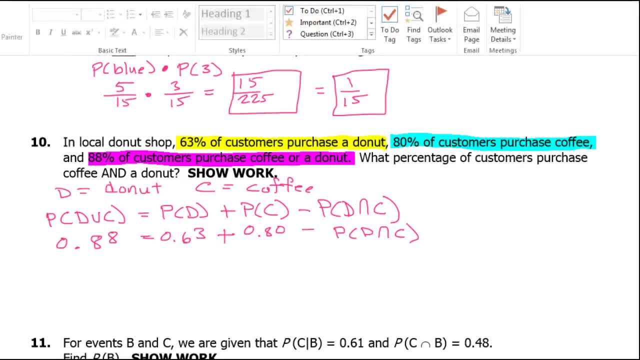 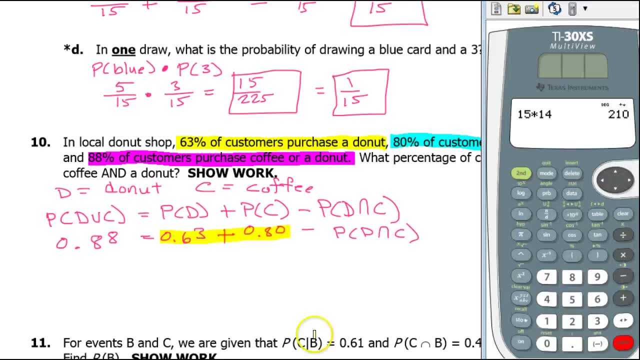 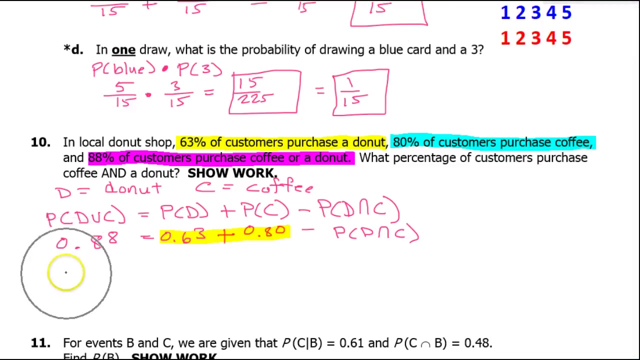 All right now if I combine my like terms. Okay, so these are like terms right here. If I put those together, All right, that's 1.43.. And in fact I'm going to write it like that. 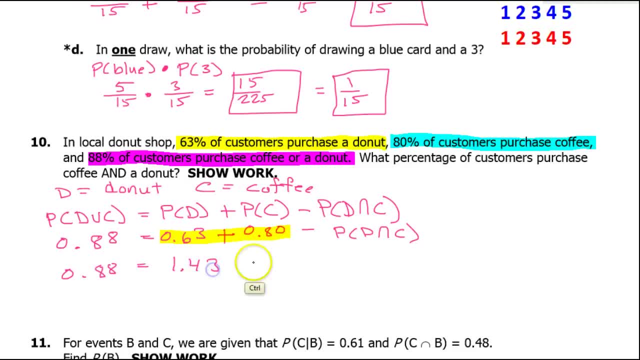 Because I'm gonna have to subtract this from 1.43 from both sides. Okay, So that's the probability of D, And if I subtract 1.43 from both sides, I'm going to leave this out. So, of course, if I want to get the probability of D and C by itself, 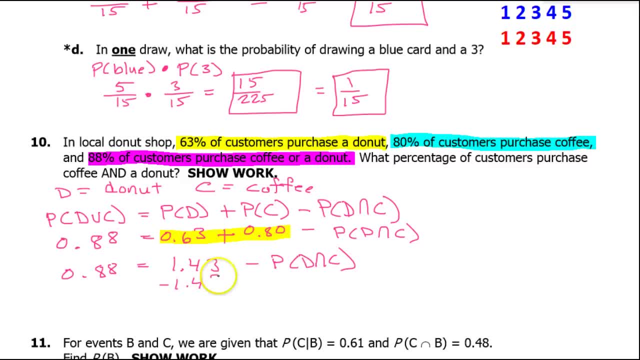 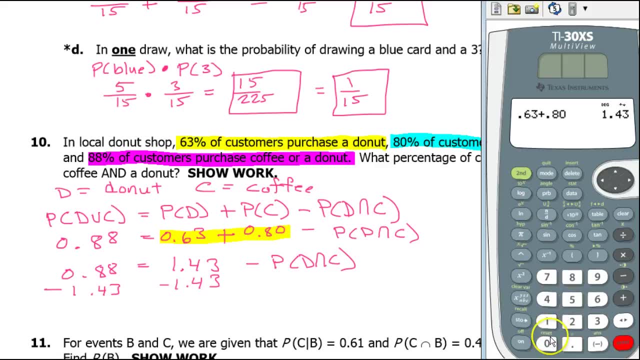 I need to subtract 1.43 from both sides, So I want to get the probability of C and C by itself. This is just some drawing And I'll have to go back to the table. Okay, so that's negative 0.55.. 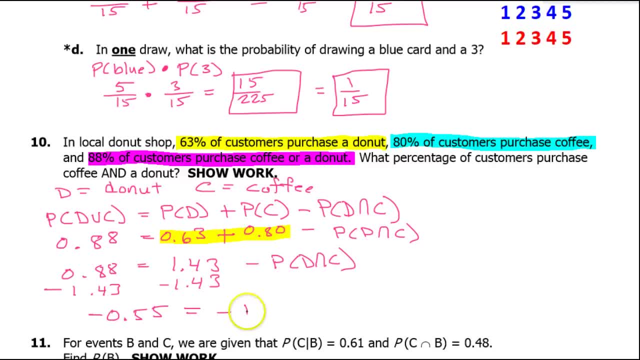 Okay, do not ignore the negative in front of this probability. This is negative probability of D and C. Now I don't want the negative probability, I want the regular probability. So I need to divide both sides by negative 1.. 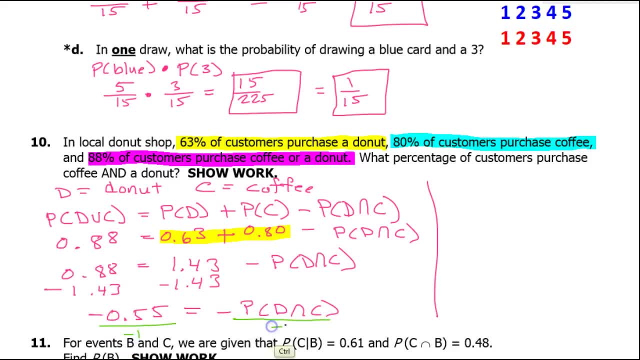 Alright, so I'm dividing by negative 1, and I'm dividing by negative 1.. So that will give me the final answer. The probability of D and C is equal to positive 0.55.. Okay, which is the same thing as 55%. 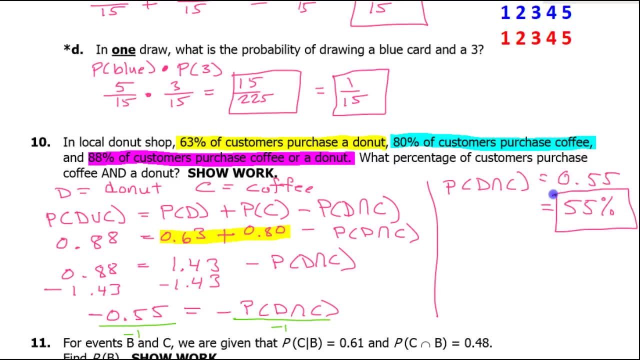 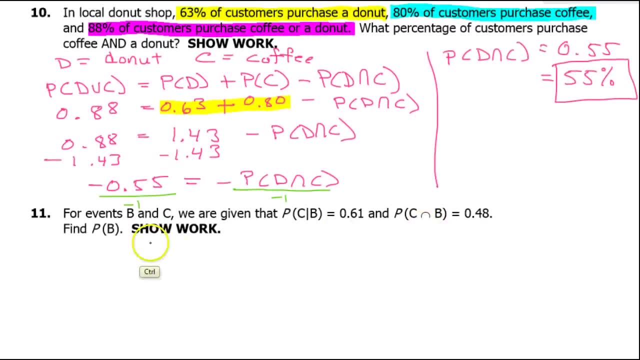 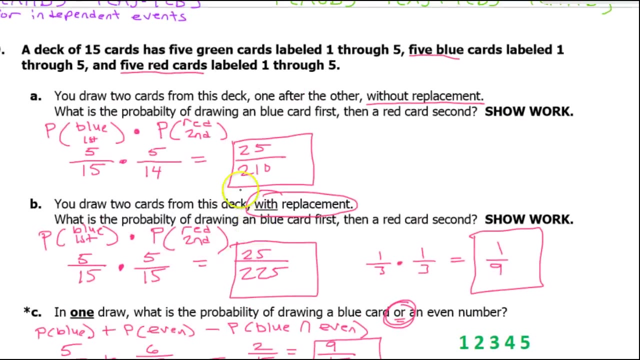 Okay, let's do one more. Alright, for events B and C. we are given all this information. Okay, notice the given part right here. C, given B: That tells us that we're going to be using the given formula shown here in red. 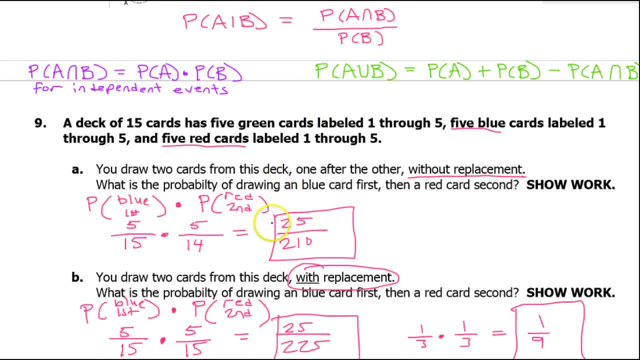 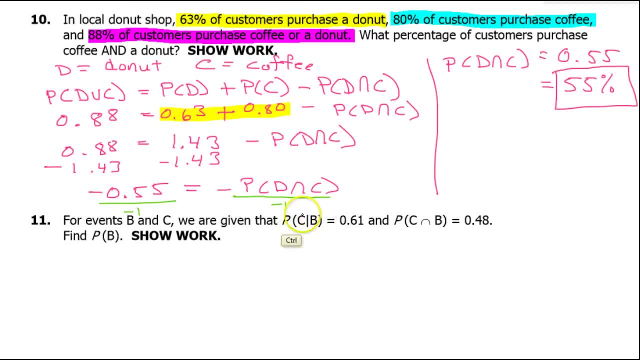 Alright, so we're going to be using the given formula shown here in red. Alright, so I'm going to use the same formula, but instead of A's and B's, I'm going to be using C's and B's, So the given formula becomes this: 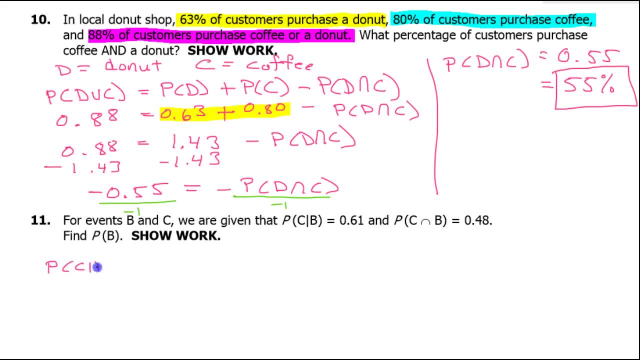 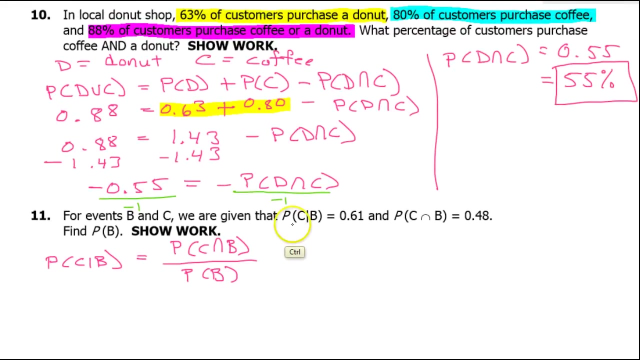 The probability of C given B is equal to the probability of C and B divided by the probability of B. So let's substitute in what we know. So we know the probability of C given B, That's 0.61.. So 0.61 equals. 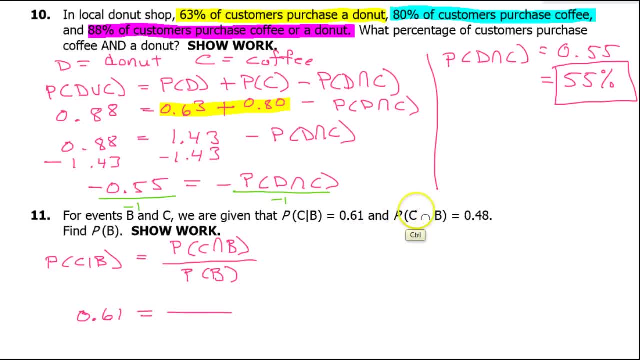 the probability of C and B. the numerator, We know that That is 0.41.. 0.41.. 0.41.. 0.41.. 0.41.. 0.41.. 0.41.. 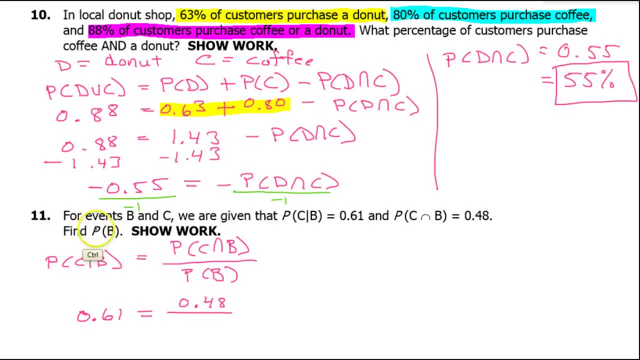 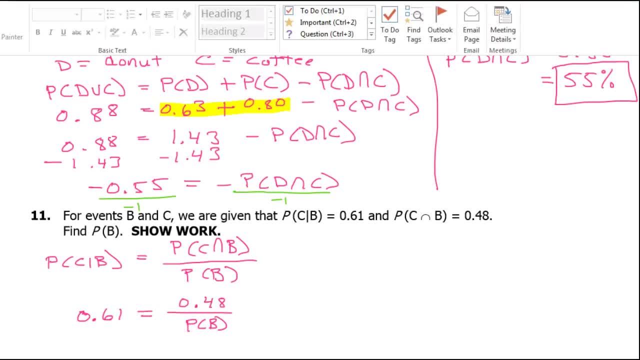 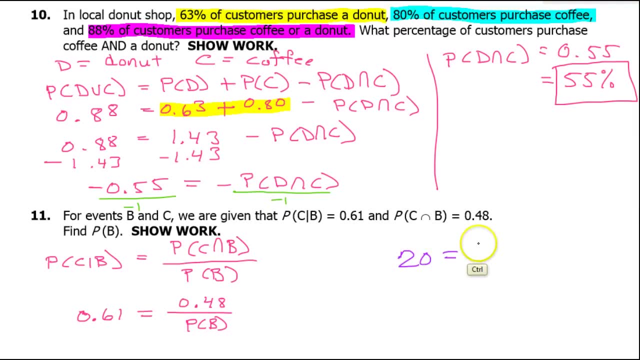 Now look here's a little off to the side reminder. When I have equations like this, like say, if I have 20 is equal to 5 over X When the variable is in the denominator, the quickest thing to do is remember that we are allowed to swap. 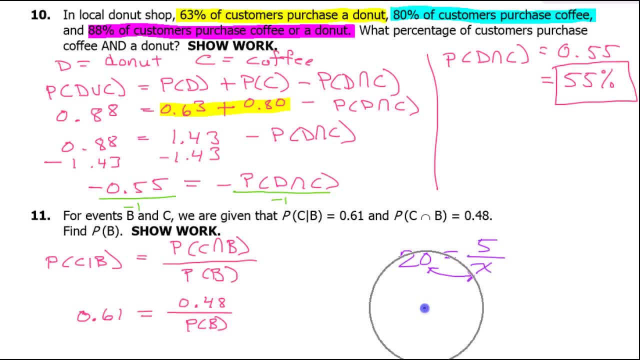 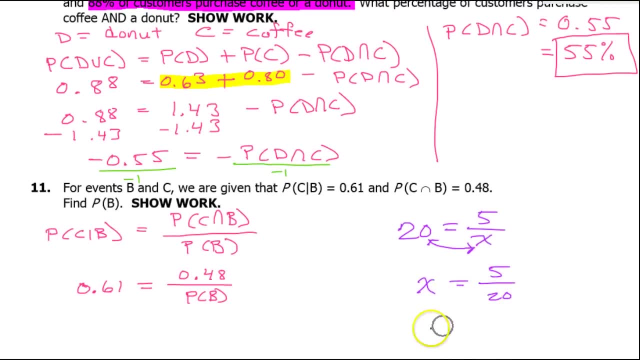 the denominator. So if I swap the 20 and the X, then I have X is equal to 5 over 20,. all right, And that's the answer. I mean, I could reduce it and put 1 over 4 if I wanted to. 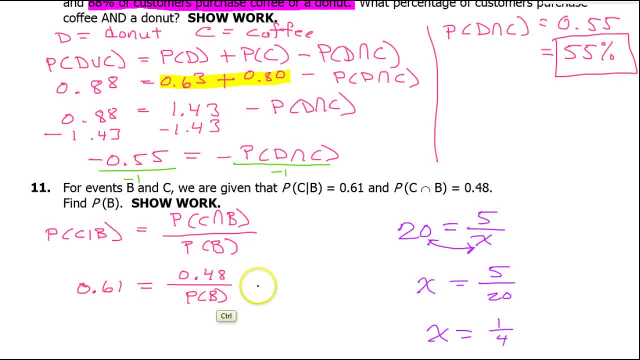 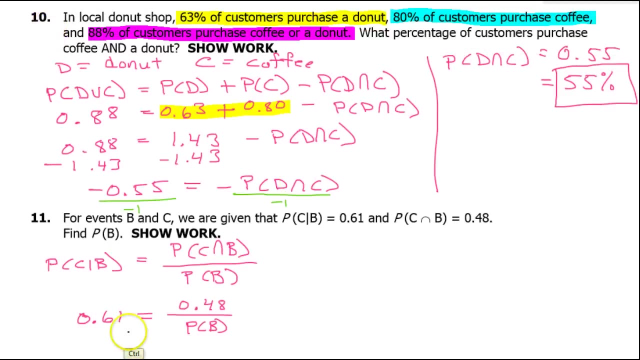 So that's what we're going to do now. Just like I can swap the 20 and the X, I can swap the probability of B and the 0.61.. So that's the quickest thing to do. All right, so if I swap these I get the probability of B is equal to 0.48 over 0.61.. 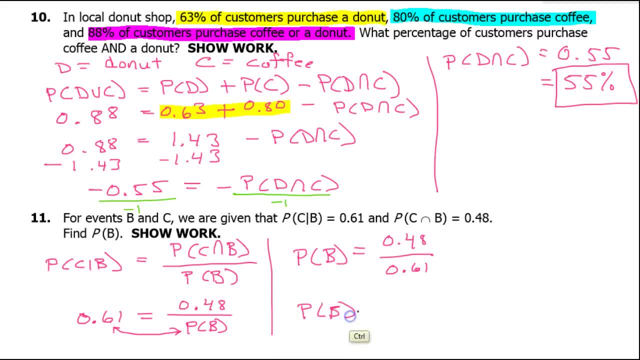 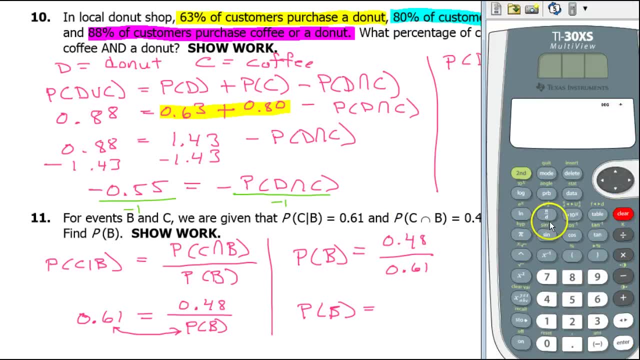 All right, do not leave it like that, With decimals inside of decimals. Go ahead and divide this out. So I have 0.48 divided by 0.61.. Okay, so I get that 0.7869.. 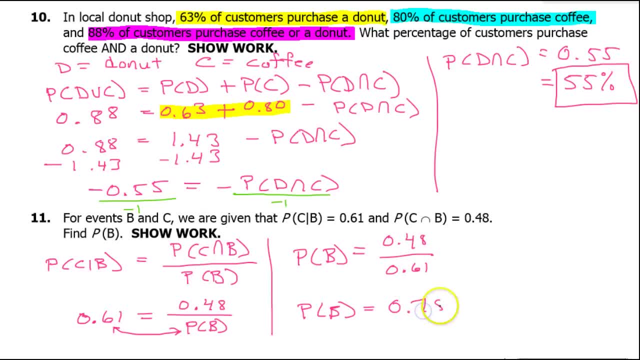 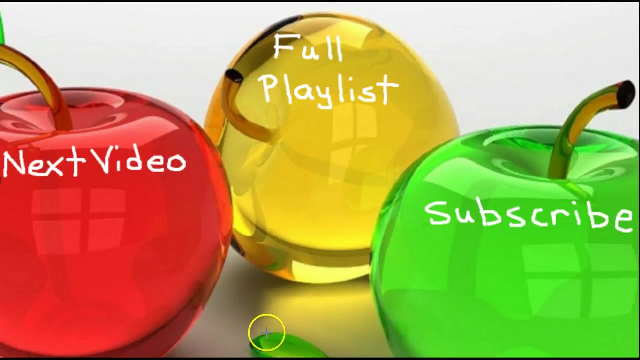 Okay, Which is approximately equal to 78.69%. All right guys, that's going to do it for this video. Go ahead and click here in the red apple to watch the next video. Click in the green apple to subscribe, or click the yellow apple for the full playlist. Thanks for watching.